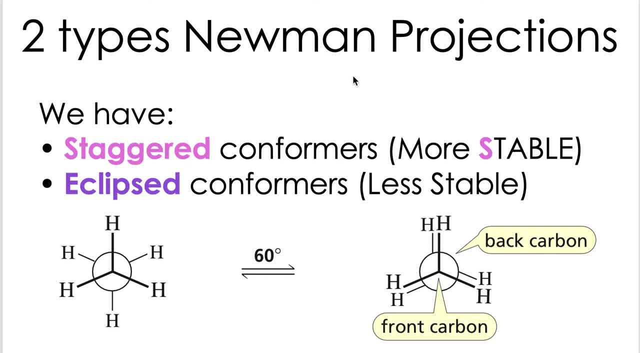 So we have two types of Newman projections. We have the staggered type and we have the eclipse type and they're called conformers because they are Newman projections. So with the staggered type we say that they're more stable- S for staggered, S for stable. So that's how I remember that. 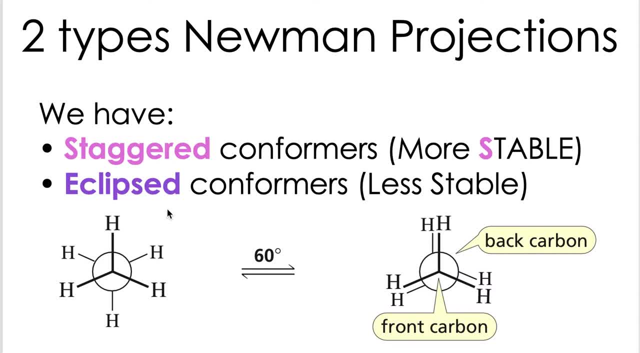 With the eclipse those are opposite of the staggered, so we say they are less stable. So over here we have a staggered conformer and over here we have an eclipse conformer, And with the staggered. so they look like this: right, we can go to an eclipse conformer from a staggered conformer. 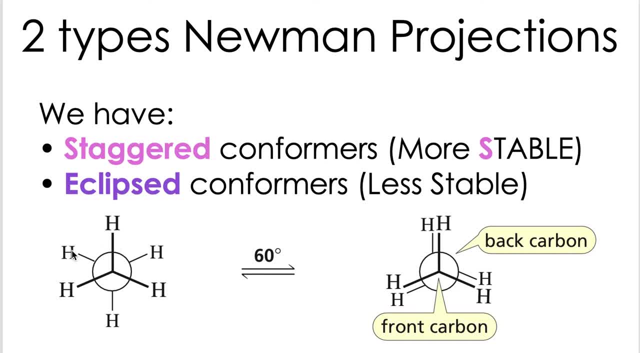 So we would rotate it 60 degrees. the hydrogens in the back right, these are the hydrogens that are in the back. So we rotate that 60 degrees and those hydrogens in the back would go behind the hydrogens that were in the front. 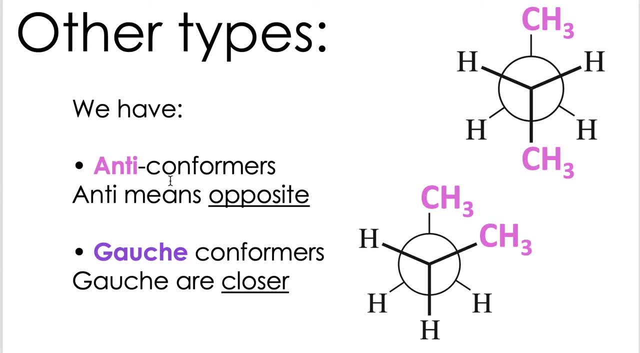 So we have other types, we have anti-conformers and we have gauch, conformers or gauch. you can say: And with the anti-conformers, anti means opposite, that root word means opposite. So let's look at this. so these are methyl groups, right, they're substituents. we call them. 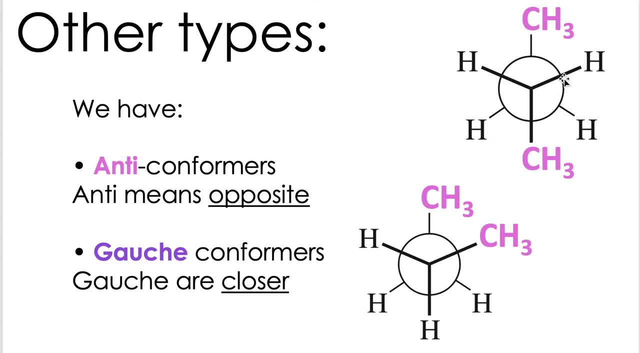 and they're placed directly opposite of each other. they're far away. directly opposite, and opposite means anti right, So anti-conformer this would be called, and it makes sense because it does look like that With the gauch conformers. gauch, we say they're closer right. so over here, the methyl groups. they 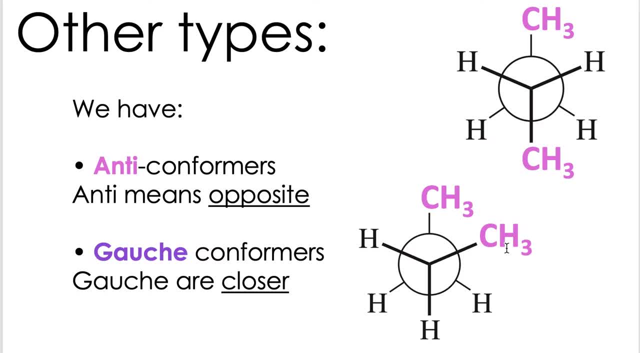 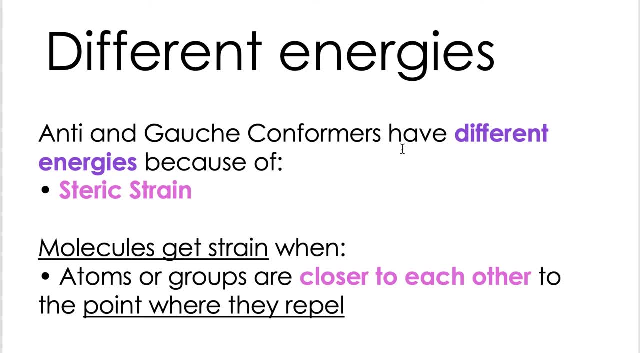 are closer to each other. so it is definitely considered a gauch conformer And they have different energies. so the anti and gauch conformers have different energies because of something called steric strain. So molecules they'll get that strain when they're closer to each other. 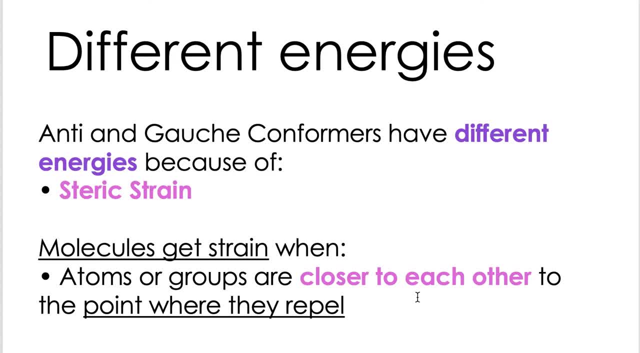 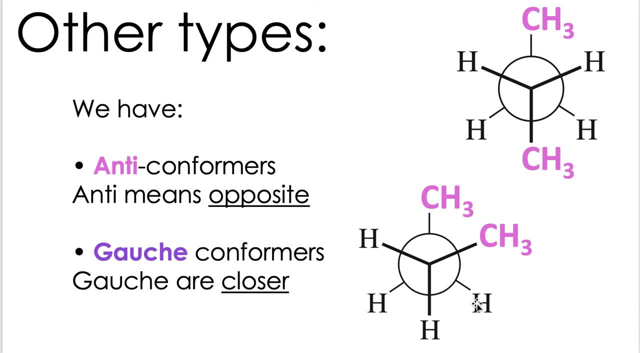 to the point where they're going to repel, because things that have like charges repel from one another. So over here we have a gauch conformer and we have anti-conformers and we have gauch conformers. Over here the gauch has gauch interactions. we say right, because these are so close to each other. 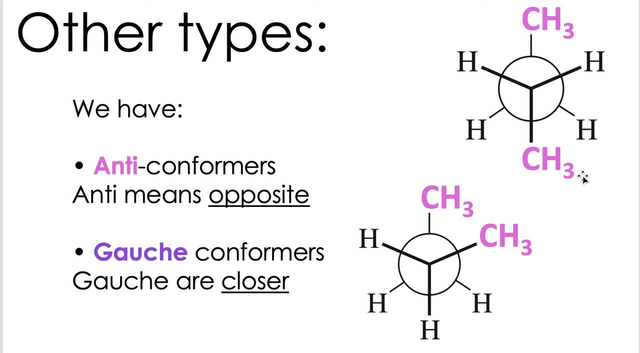 that they're going to want to repel or move away from one another. Over here we don't have as much steric strain because they're completely opposite each other and they're far away.